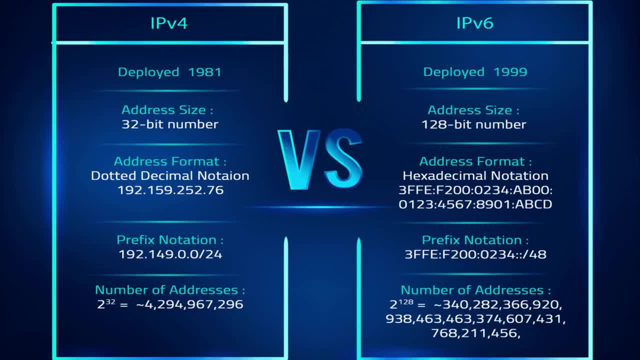 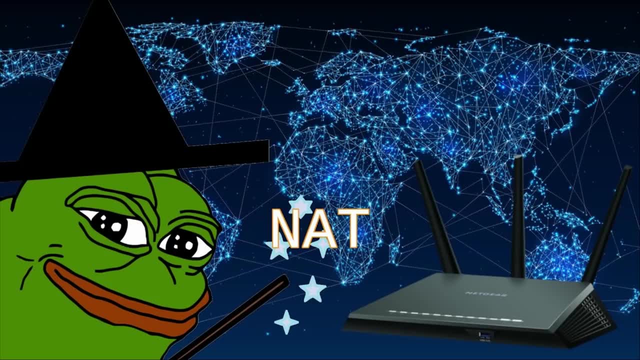 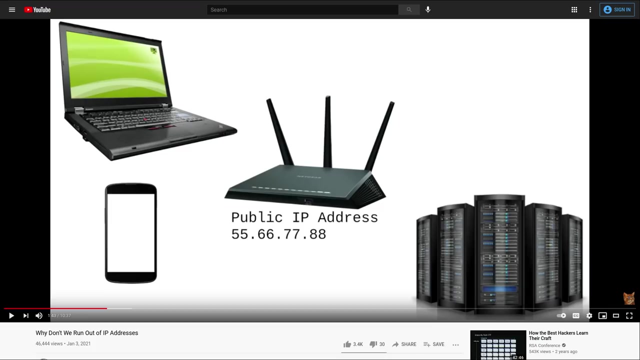 realized that the world was quickly running out of IP addresses. There were some solutions to slow the hemorrhaging of IP addresses before IPv6 could be completed, like network address translation, which essentially allows multiple devices that are on a single LAN to access the internet without each of them needing their own public IP address for it. You should check out. 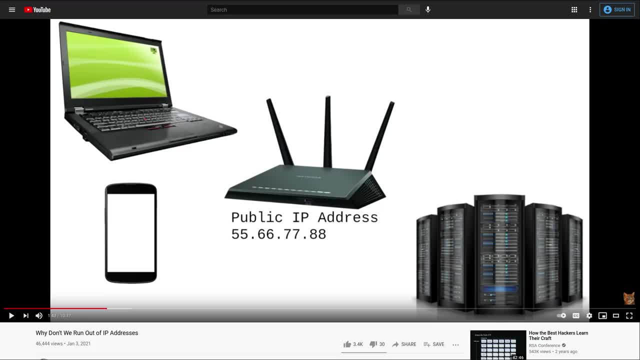 my video on that if you're interested in the technical details of NAT. But with IPv4, it's unlikely that we'll start running out and need to do anything anytime soon to start conserving them, because IPv6 is a 128-bit address. That means that with IPv6, there are 2 to the 128 possibilities. 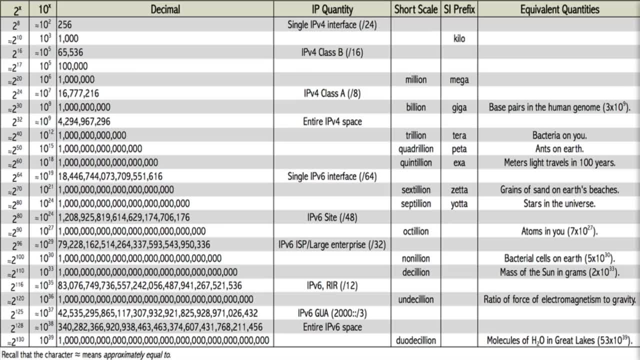 or 340 trillion trillion trillion possible addresses. So to put that in perspective, the estimated number of bacteria on earth is 5 times 10, to the 30. So if each individual bacteria had 1 million smartphones, smartwatches, whatever kind, 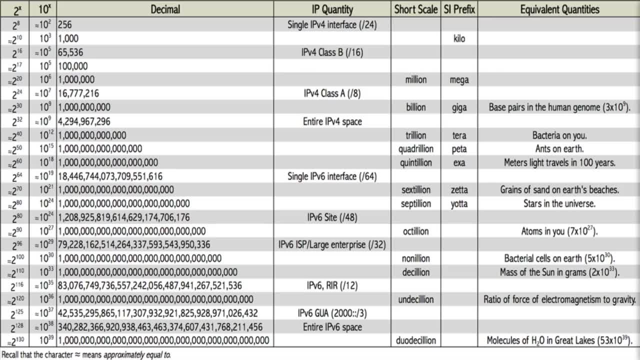 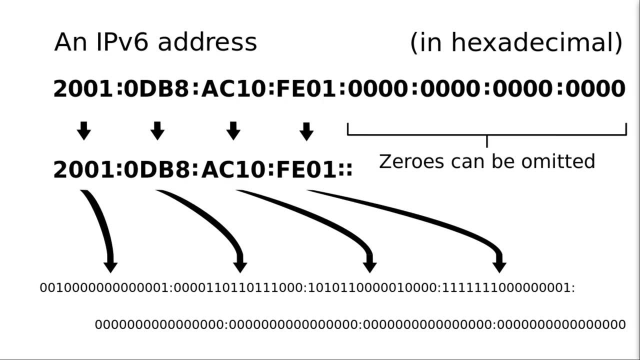 of device can connect to a network. we could supply them all with IPv6 addresses and only use up less than 2% of that available address space. So this is what your standard IPv6 address looks like. Quite a few differences between this and IPv4.. So instead of four octets, we have eight. 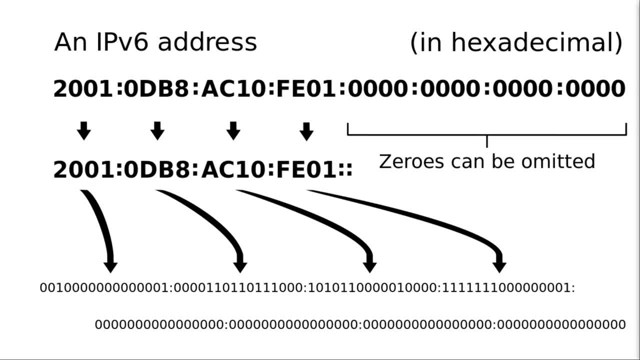 segments that are called hextets, And we have colons that are separating those hextets instead of dots, like we see with IPv4's octets, And each digit in the hextets are done in hexadecimal, which is probably where the 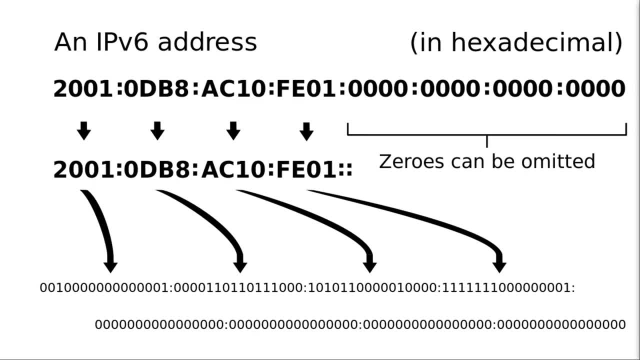 name comes from, So the value of each digit can be zero through F. These addresses are really long and they get even longer when you translate them into binary, because each value is going to represent four bits. So, for example, this 2 would be 0010.. Each of these zeros would just be four zeros in binary. The 1 would be 0001.. 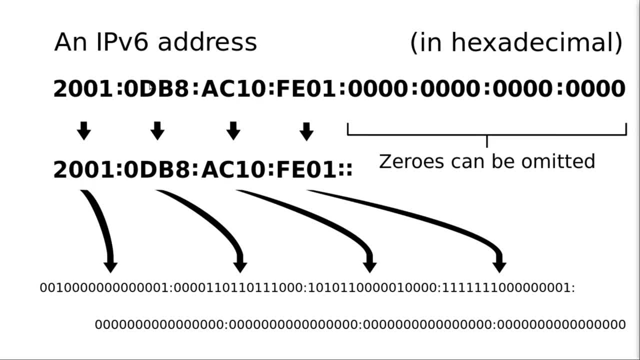 We already know what that zero is going to be. Now. the D represents 13 in base 10.. So if you counted out 0 through 9,, then A is 10,, B is 11,, C is 12,, D is 13.. And so in binary that would be: 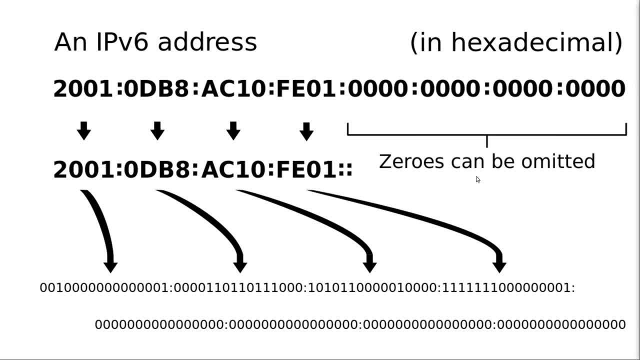 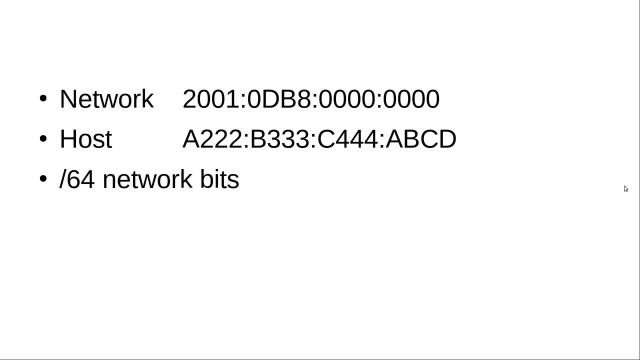 0.. So it's important to understand how this hex to binary conversion works, to understand the IPv6 subnetting. So subnetting is also pretty different with IPv6. So there is a network and a host section of IPv6 addresses, just like IPv4. But typically an IPv6 address is going to be split. 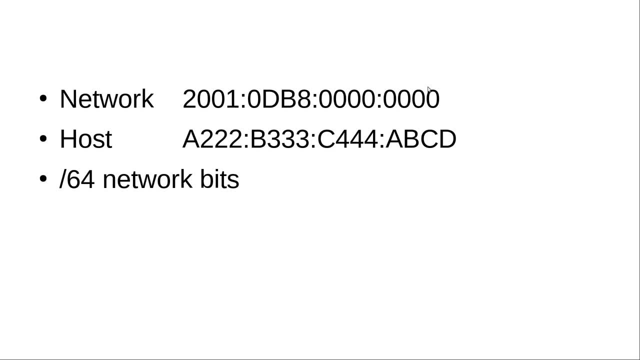 right down the middle, where the front half is the network part and the second half is going to be the host part. But IPv6 does not use a subnet mask, So instead you just write a dash and the number of network bits, which in this case is going to be 64 bits, And, if you haven't noticed already, 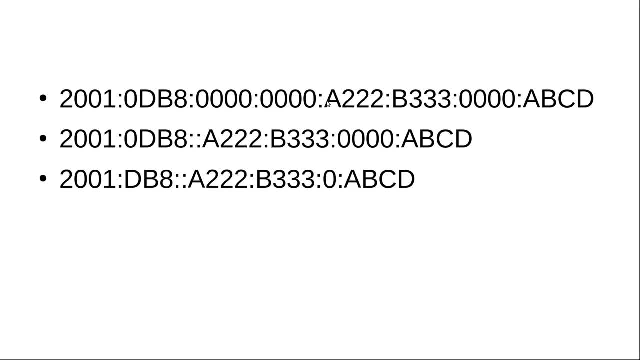 this address. it is pretty obnoxious, It's very long and nobody is going to want to type that out again and again, So let me show you some ways that you can shorten it. So the first trick is to remove groups of zeros. You're going to get this a lot in. 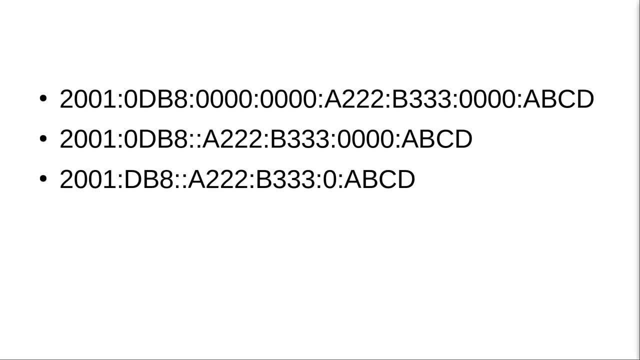 IPv6 addresses because there's just so many of them, We usually don't need all of the hextets to get an available, usable address. So very often you're going to see several of the hextets be all zeros And when that happens you can just compress them into a single- well, into a double. 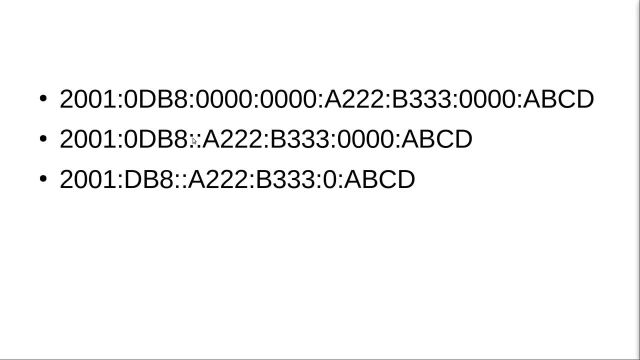 colon. like you see here Now, you can only do this once with all of the groups of zeros that are next to each other, which is why these four zeros are going to be all zeros. So you can just run it over and over again, and over again until you get an exact value of that. 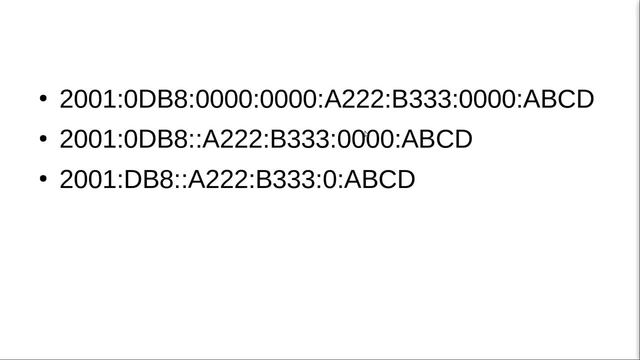 So here is the first group of zeros. Over here you can see all of the hextets are all zeros. So let me show you another example of a double colon. If you had more than one double colon it would be impossible to know how many groups of zeros each one had. You wouldn't know if back 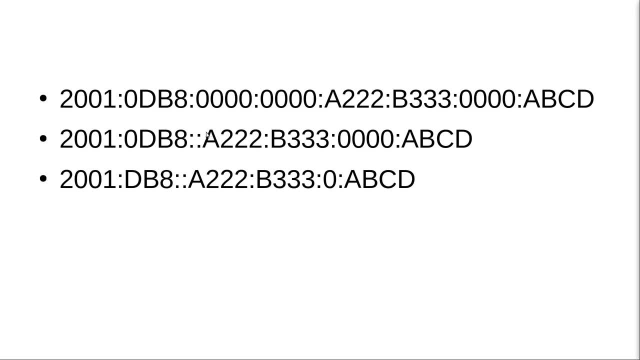 here was two groups, or over here was two groups, or this one was one group, this one was one group. It'd be impossible to know which one is which, so you can only do this once Now. another trick is to remove all of the leading zeros from each hextet, So I took out the zero key. it's about 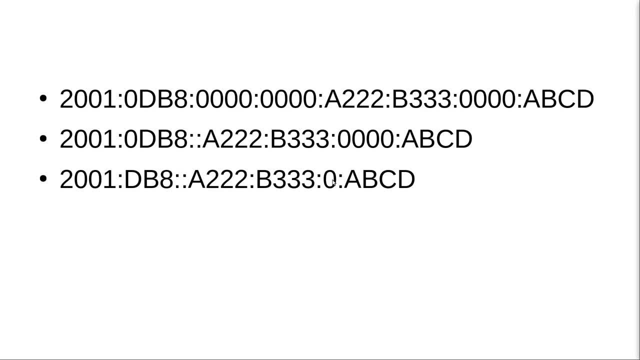 here from 0db8 and over here there were three leading zeros, so I can just compress this whole thing down to a single zero. and there you go. so this is quite a bit shorter. this is maybe two thirds of the size of what we started with in our ipv6 address and, like I said, there's going to be. 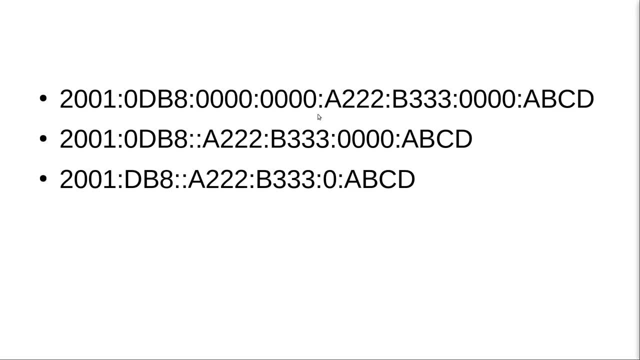 a lot of them that have several hextets, that are all zeros. so you can imagine there's going to be a lot of situations where you can shrink this down a whole lot, maybe get it down to half of the size of what this is. now again, just like ipv4, there are ipv6 addresses that are designated for. 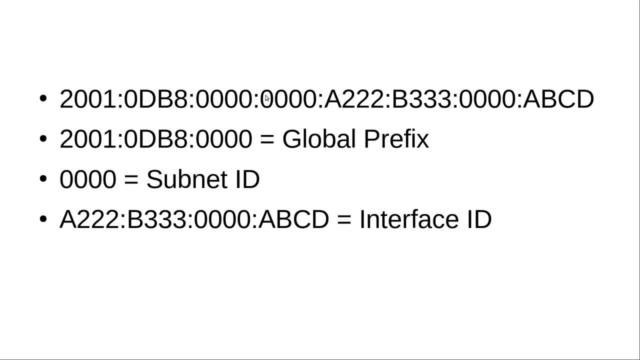 specific purposes. so far, what we've been looking at is a global unicast address which essentially has the same purpose as an ipv4 public address. but there's no reason at all for all those different devices to just use one public ip address because, again, we have so many of them. so ipv6 can give each individual device its own public ip address. 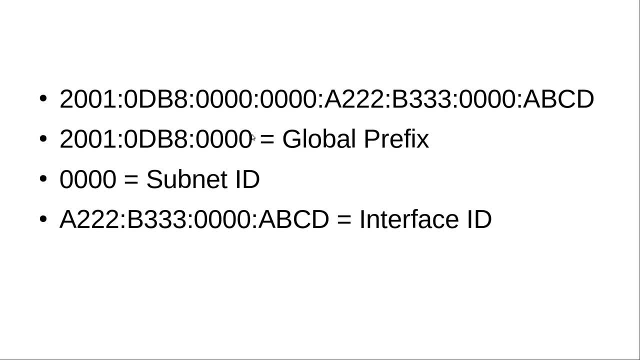 so the first part of this address is the global prefix, which will always be 48 bits or more, and it's what your isp is going to provide you with: a block of ip addresses. then, next, we have our subnet id, which has 16 bits, which gives us over 65 000 possible subnets, and, of course, 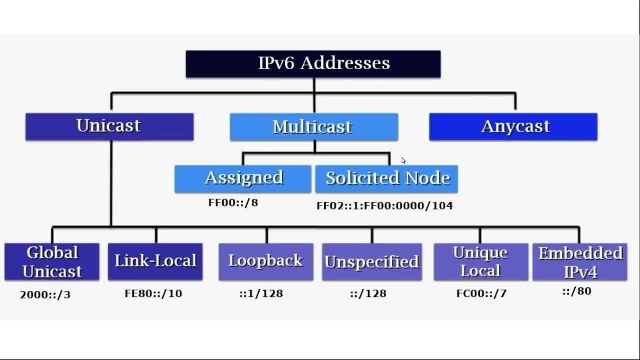 we're going to be looking at some of the other ipv6 address types, so we've got link local addresses which are not globally routable. in fact they aren't routable at all. they are used for addressing on a single link. they're primarily used for things like neighbor discovery, and they are the first. 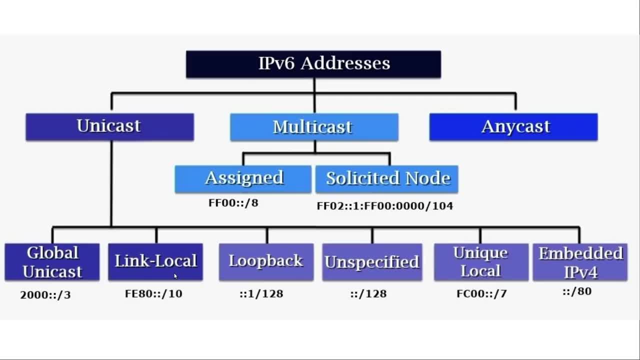 addresses that are created on an interface before an ipv6 router has time to advertise all of its routes. they are designed to communicate with a single link. so we're going to be looking at some of the other ip addresses that are created on an ipv6 router. so we're going to be looking at some. 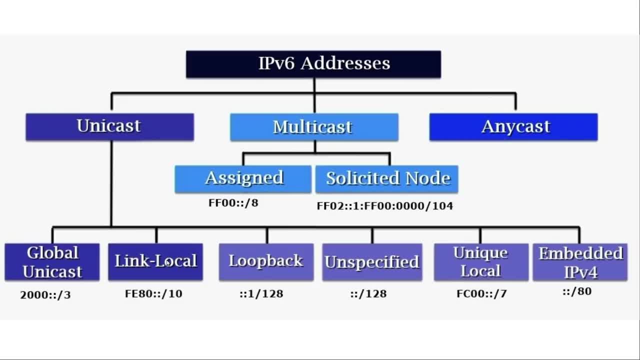 area of a network not separated by any routers. it's pretty similar to the automatic private ip addresses that you see in ipv4 that begin with the 169.254 addresses. if you've ever seen those you know what i'm talking about. so, similar to those and its prefix is fe80, colon, colon forward. 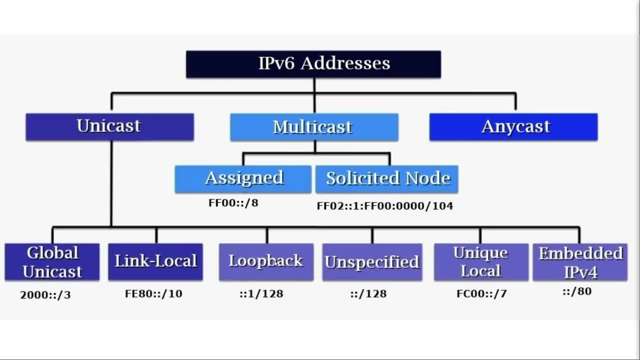 slash 10.. so then we have loopback. that's going to be the same concept as ipv4 loopback, so it's used for testing the functionality of your network card without needing to actually connect to a network unspecified. this indicates the absence of an address and one. 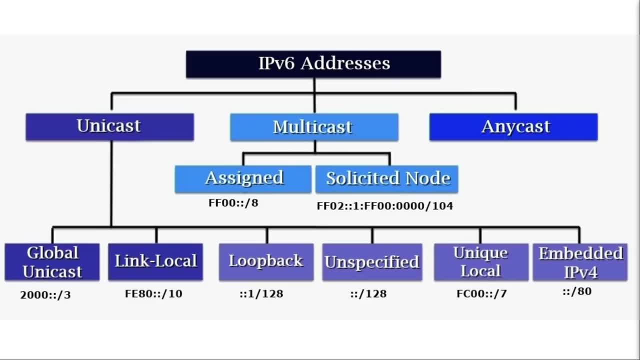 example of its use is in the source address field of an ipv6 packet that's sent by an initializing host before it is learned its own address, this is going to be written as all zeros, so every single one of the hextets is all zeros. that's why. 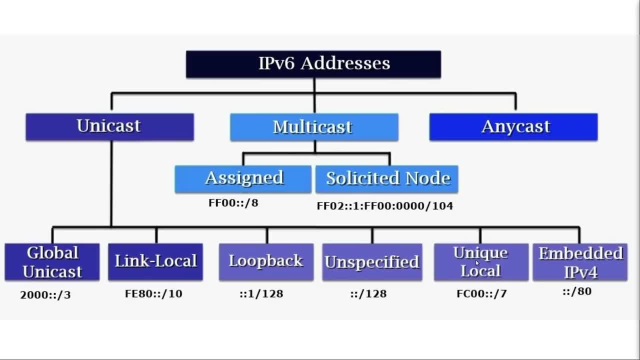 you can shorten it to just this double colon here: unique local. that's similar to an ipv4 private address, so it's not globally routable, it's just going to stay in the LAN. you know, whichever one router or couple of routers is in your organization, the prefix to identify it is: 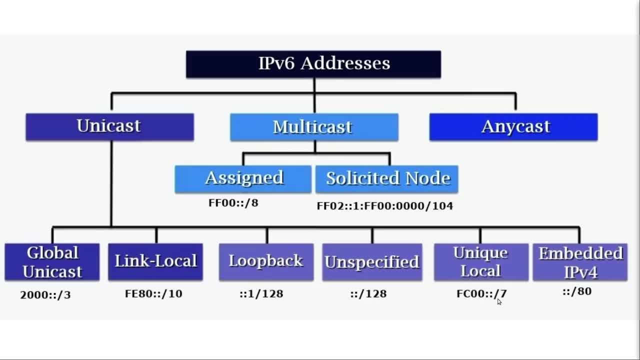 fc00 double colon forward slash seven. embedded ipv4 is used to represent the ipv4 address space within the ipv6 address space. so now it's pretty easy to do. considering how much larger ipv6 is than ipv4, obviously it can encompass all of that space and have many 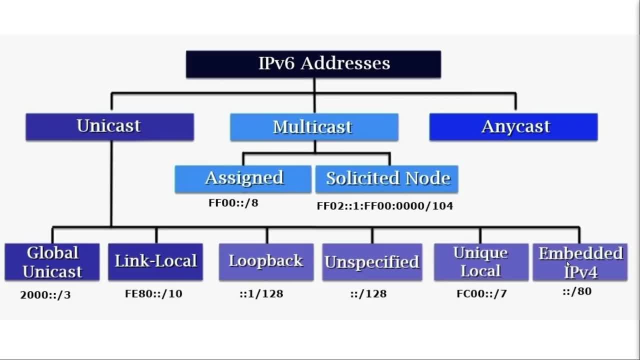 many more left over. that's mostly going to be used internally with apis and operating systems for ipv4 to ipv6 compatibility, multicast addresses are sent to a group of devices that are running for that particular multicast address and they are essentially an upgrade to ipv4's. 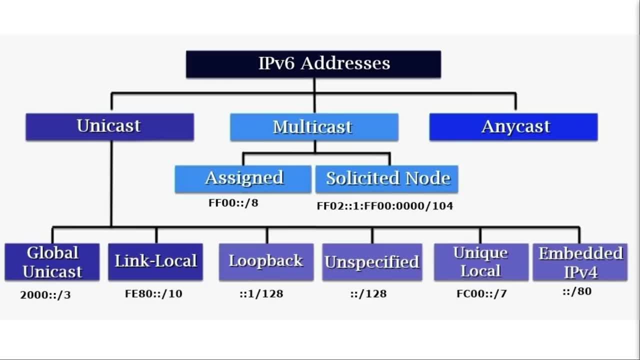 broadcast address, because they don't force every single device to process the packet. so this is going to be especially useful for any type of low-powered devices, things like embedded devices, which may be on a network running in a low power mode, and so the network interface is able to.